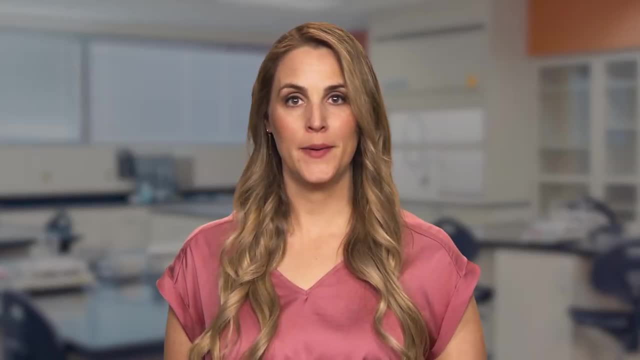 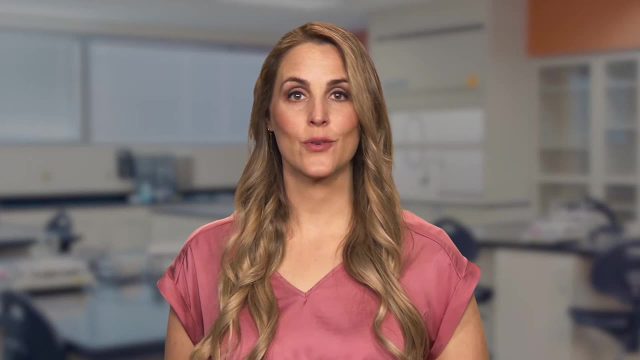 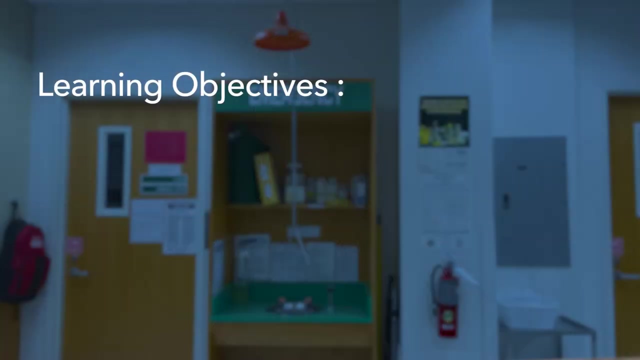 In the lab. safe behavior and appropriate PPE are key to preventing personal exposure to hazardous materials. However, in the event that your eyes or skin are exposed to hazardous chemicals or biohazardous materials, you should know what to do. The purpose of this video is to demonstrate how to use the safety. 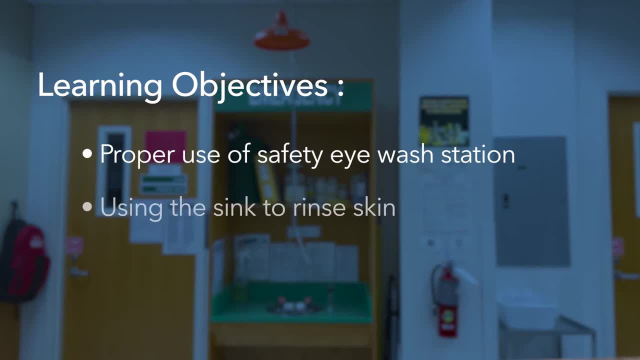 eyewash station in the event a material gets in your eyes, how to use a sink to rinse skin in the event of a small skin exposure. and how to use the safety shower in the event of a large body exposure. Note that safety showers and 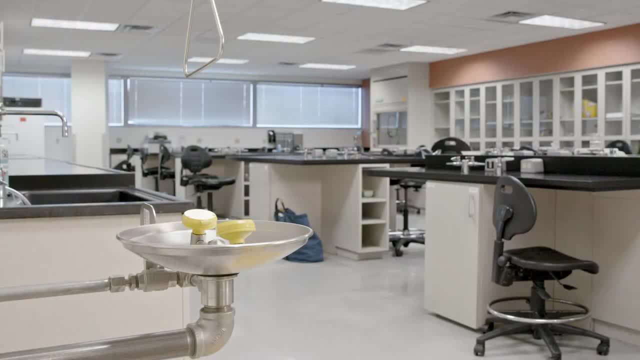 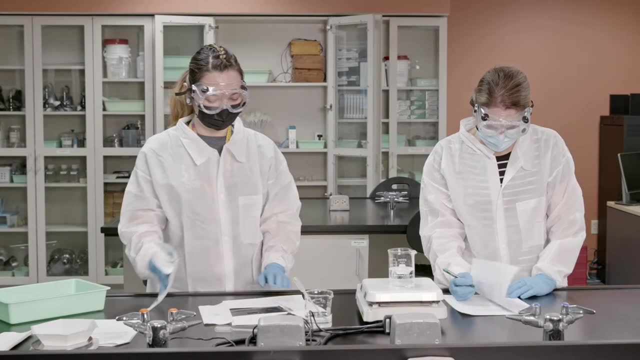 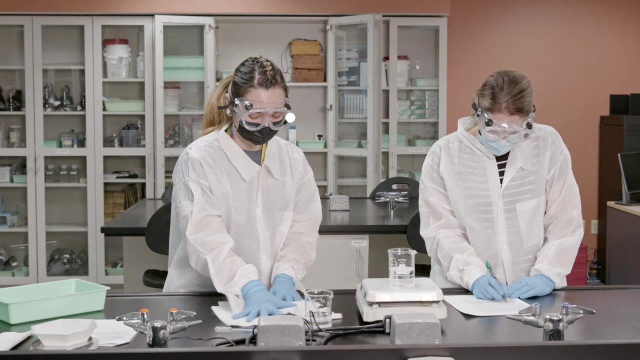 eyewash stations may look different at different campuses. You will see the equipment used at your campus during your on-site lab safety orientation. For true splash protection, only wear safety goggles marked with the ANSI Z87 plus D3 designation and wear goggles for the entire. 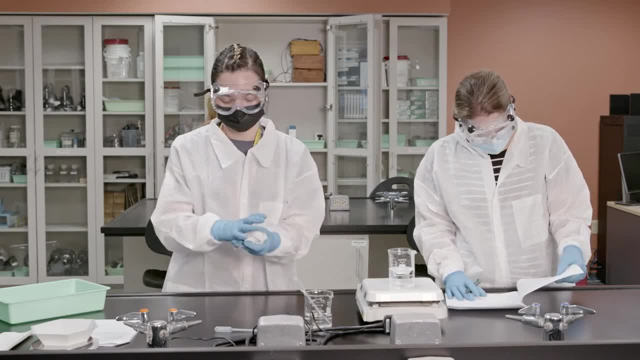 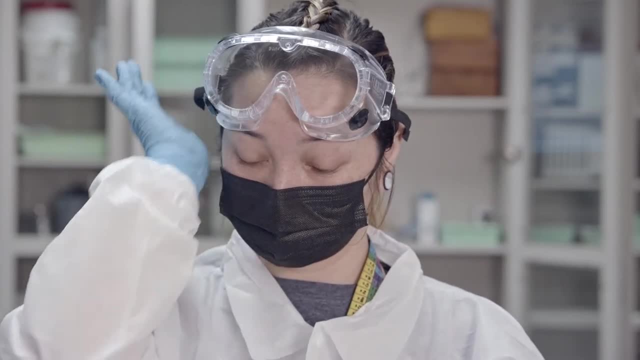 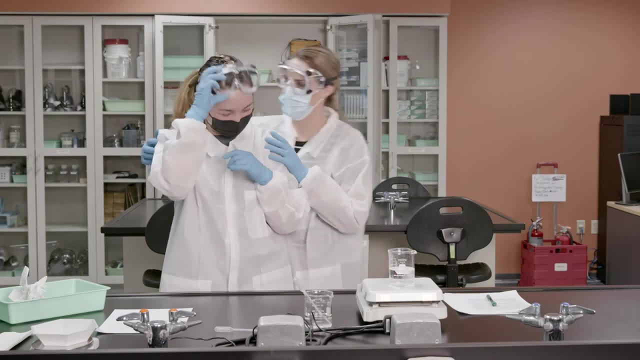 lab. Also, never touch your eyes while in the lab, as your hands may be contaminated with a chemical. In the event that a chemical or hazardous liquid does get into your eyes, proceed immediately to the nearest eyewash station. It may be difficult to see, so ask someone for help. Most eyewash stations have a lever or 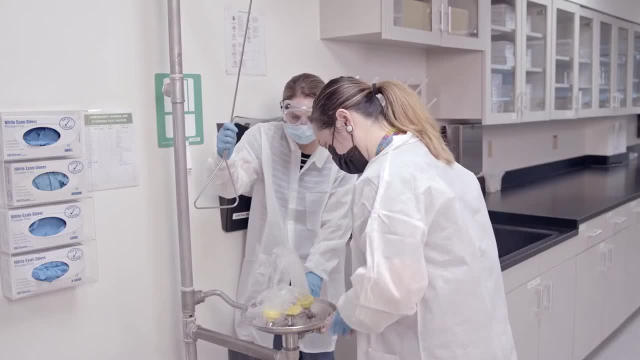 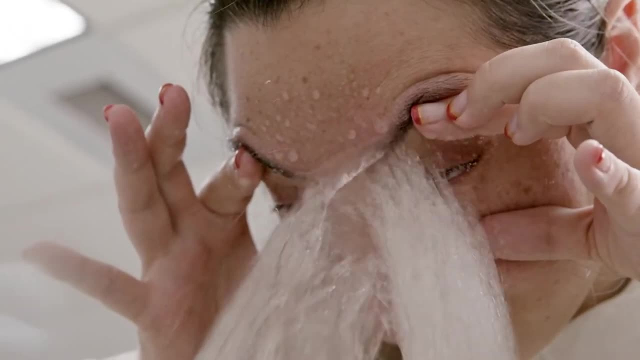 handle to activate the water flow. Activate the water flow and place your eyes directly in the water. You will need to hold your eyelids open and let the water wash your eyes for 15 minutes. It will not be comfortable to hold your eyes open in the water for that long, but it is necessary to flush out the 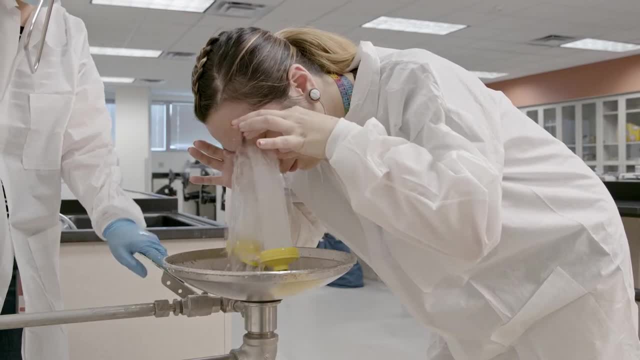 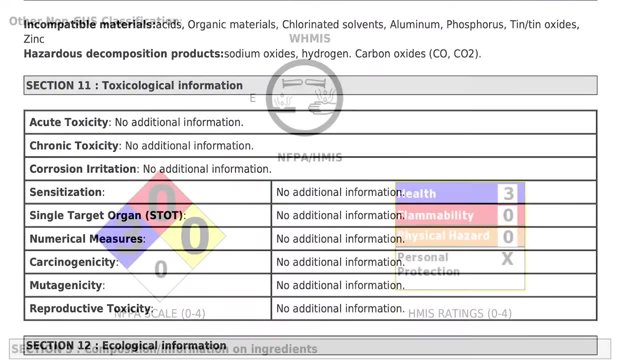 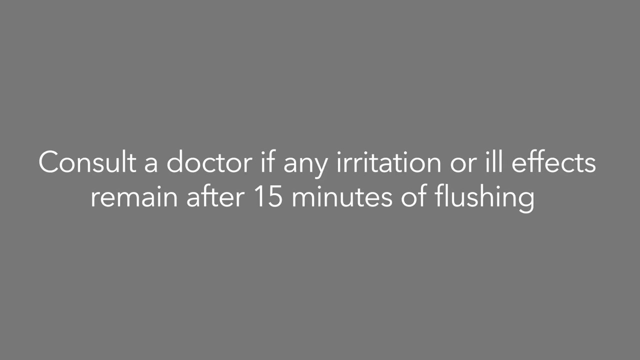 hazardous material and it is well worth it to save your eyes. Have someone call security and check the SDS for the material that was splashed in your eyes. Ensure that security documents the incident with an incident report. afterward Consult a doctor if any irritation or ill effects remain after. 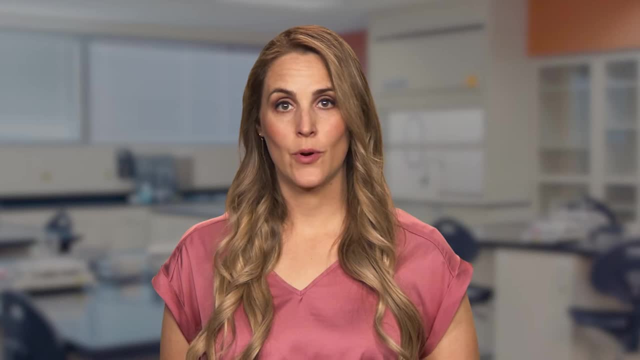 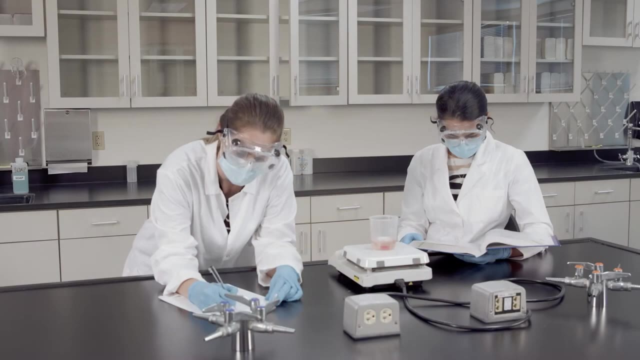 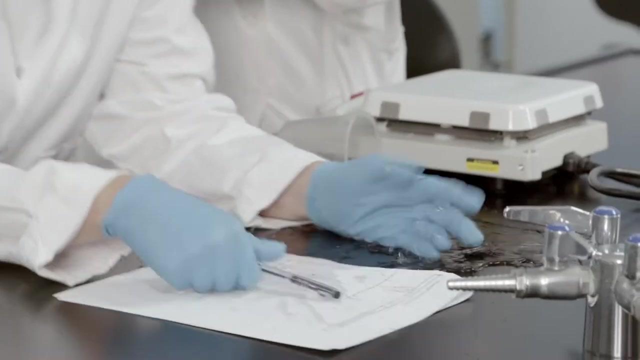 15 minutes of flushing. It is possible that you will spill a chemical or hazardous material on your skin in the lab, especially if you're not wearing protective sleeves or a lab coat. Depending on your campus or your course, lab coats may or may not be required In the event of a small splash to your arms.